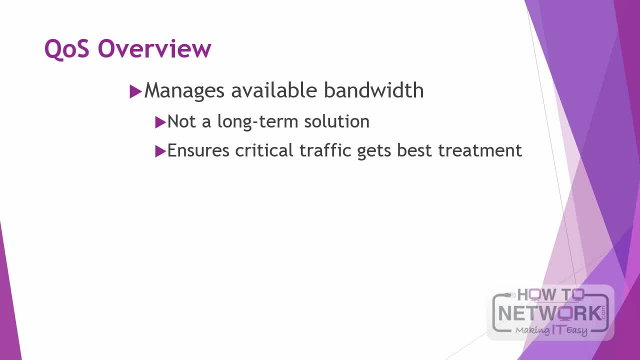 of service does not add bandwidth, but it helps you make better use of what you have. If you have chronic congestion issues, quality of service should not be the primary answer to resolving that problem. You need to add more bandwidth, However, by prioritizing traffic. 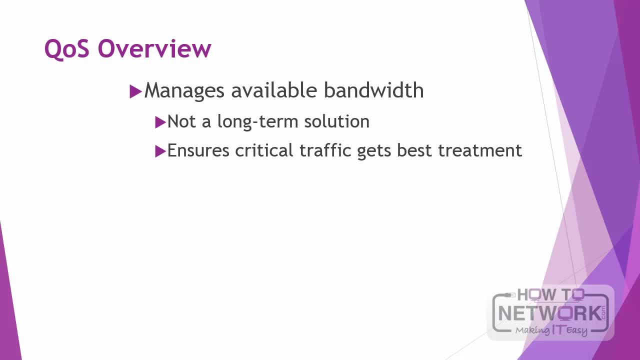 using quality of service, you're going to be able to reduce the amount of traffic that you have. Quality of service is a tool for managing a WAN's available bandwidth. You can make sure that your most critical traffic gets the best treatment and available bandwidth in times. 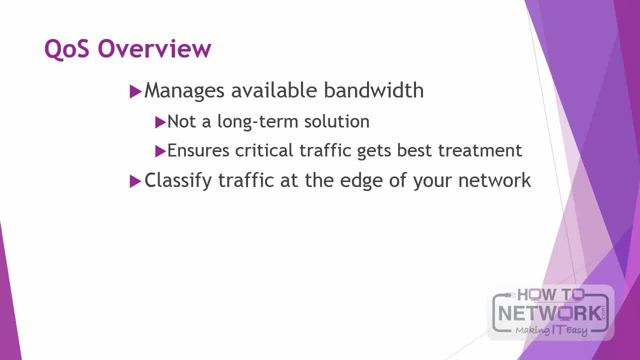 of congestion. One popular quality of service technique is to classify your traffic based on a specific protocol type or matching access list and then giving a policy treatment to that specific class. You can define many classes to match or identify your most important traffic classes, For example video or voice, And then the remaining unmatched traffic then uses a default. 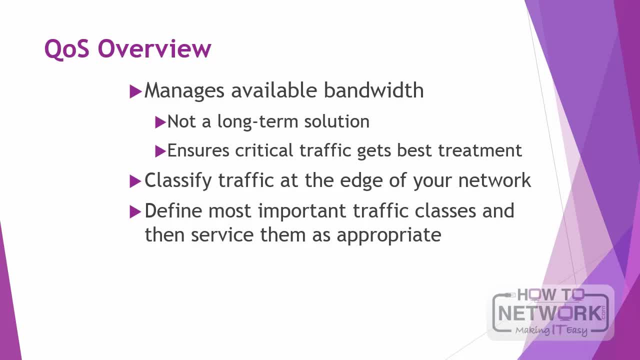 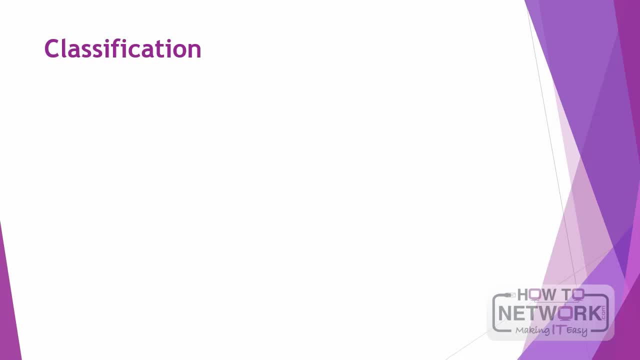 class, which is the traffic that can be treated as best effort. So let's begin with classification. For a flow to have priority, it must first be identified and marked. Both of these tasks are referred to as classification. The following are popular technologies which support classification: 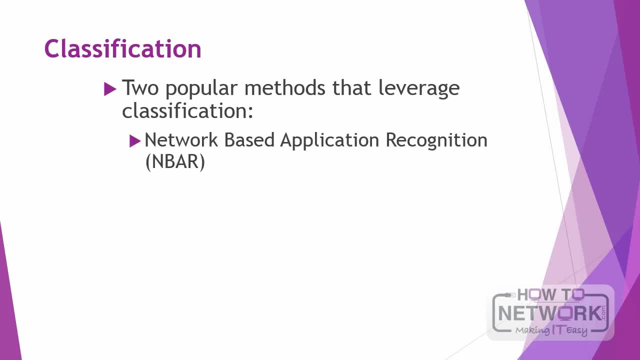 NBAR- NBAR. NBAR is a technology that uses deep packet content inspection to identify network applications. So an advantage of NBAR is that it can recognize applications even when they do not use standard network ports. Also, it matches fields at the application layer. 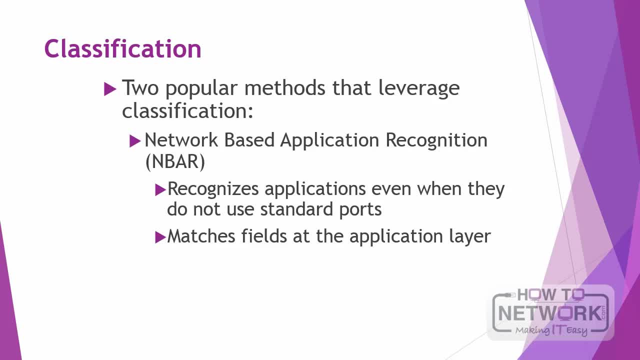 Before, NBAR classification was limited to layer four TCP and UDP port numbers, but NBAR has changed that. Next is CAR committed access rate and uses an ACL to set precedence and allows customization of the precedence assignment by the user source or destination IP address or even. 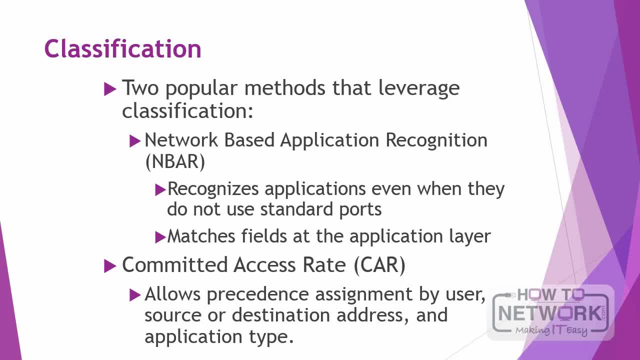 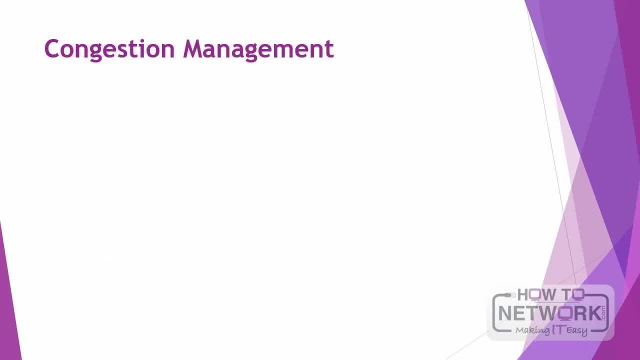 application type. Next, let's talk about congestion management. There are two types of output queues that are available on routers: hardware and software: NBAR, NBAR, NBAR- NBAR: The software queue schedules packets and places them in the hardware queue. 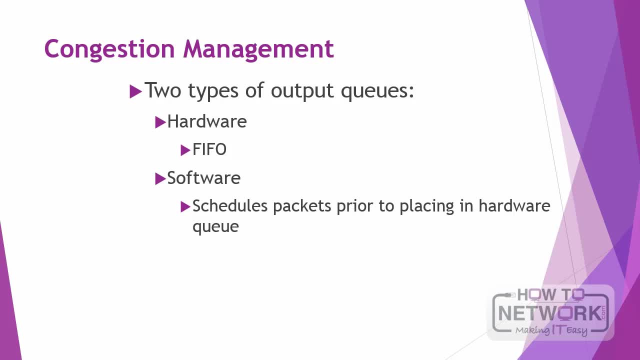 Now keep in mind that the software queue is only used during periods of congestion. before congestion. This uses quality of service techniques, such as Priority Queueing, Custom Queueing, Weighted Fare Queuing, Class-Based Weighted Fare Queuing, Low Latency Queuing and Traffic. 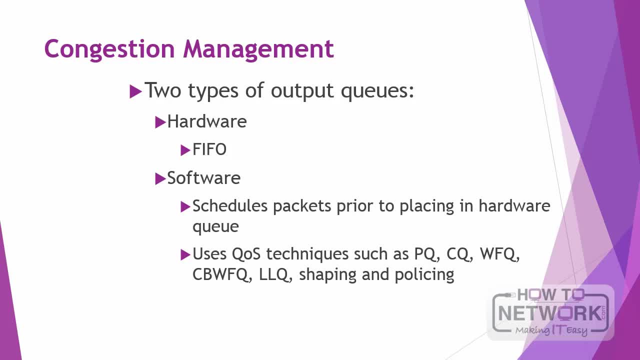 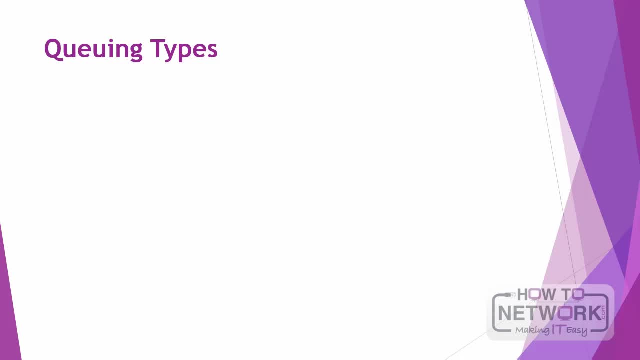 Shaping and Policing. Firstly, let's look at each of these instruments. Cisco moves the power at the alc 되 плат. not expect you to know each of these in detail again- that would be later in your CCDP studies- but, that being said, they want you to understand what each of. 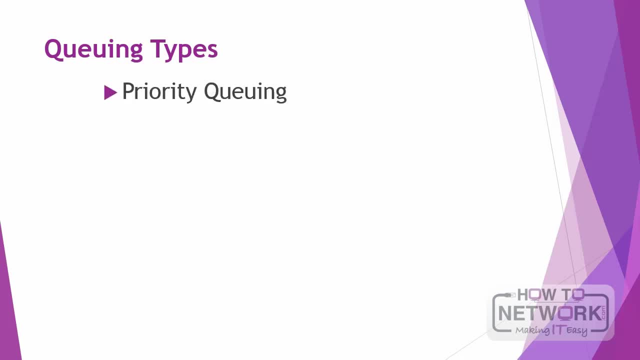 these are: priority queuing is a queuing method that establishes four interface output queues that serve different priority levels, which are high, medium, default and low. unfortunately, priority queuing can starve other queues if too much data is in one queue, because higher priority queues must be emptied first. 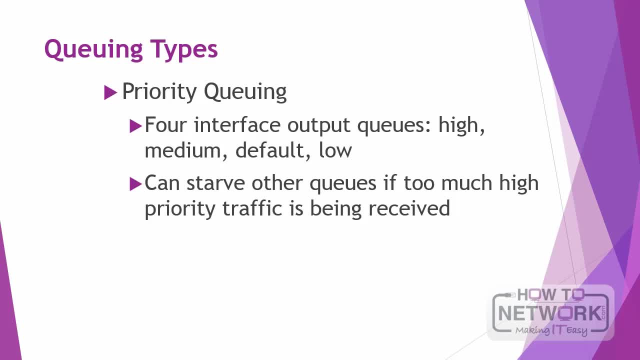 before lower priority queues. next there is custom queuing. it uses up to 16 individual output queues. bite size limits are assigned to each queue so that when the limit is reached, it proceeds to the next queue. the network operator can customize these limits and custom queuing is obviously farer than. 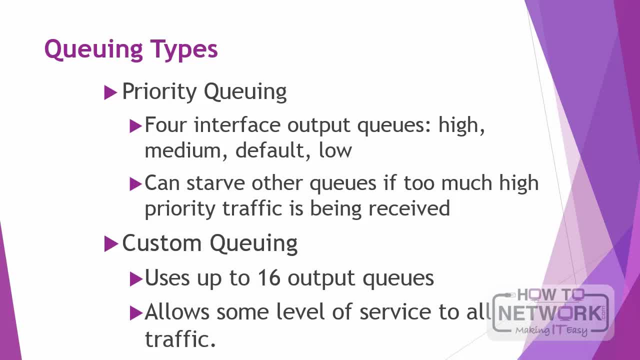 priority queuing because it allows some limit to the queue. so when the limit is reached it proceeds to the next queue level of service to all traffic. but this is really a legacy solution because there are improvements in the queuing methods which we'll talk about next. 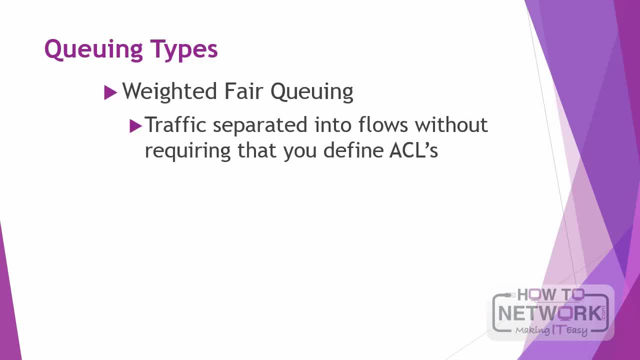 Weighted fare queuing ensures that traffic is separated into individual flows or sessions without requiring that you define access lists. Weighted fare queuing uses two categories to group sessions: high and low bandwidth. Low bandwidth traffic has priority over high bandwidth traffic and high bandwidth traffic. 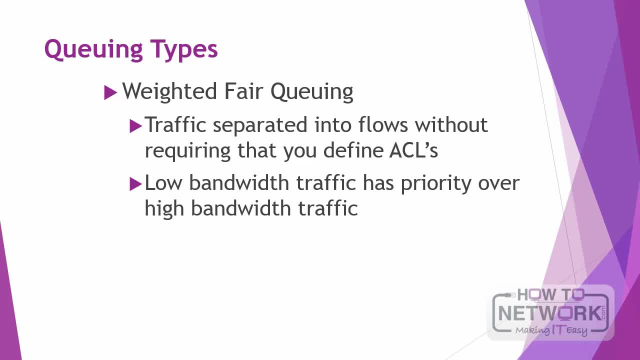 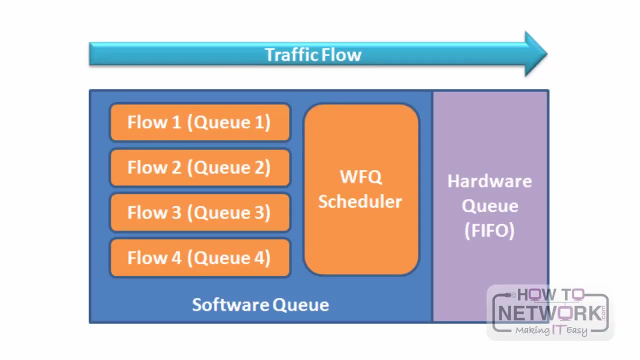 shares the service according to assigned weight values. Please know that weighted fare queuing is the default quality of service mechanism on interfaces below 2 megabits per second. Weighted fare queuing is not the best option in every scenario because it doesn't provide: 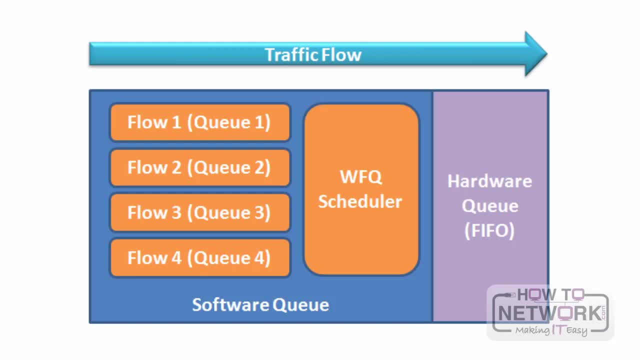 enough control in the configuration, but it is far better than the first in first out approach. This is because interactive traffic flows that generally use small packets do get the priority they need in the software queue. As you can see in this diagram, the different weighted fare queue traffic flows are placed. 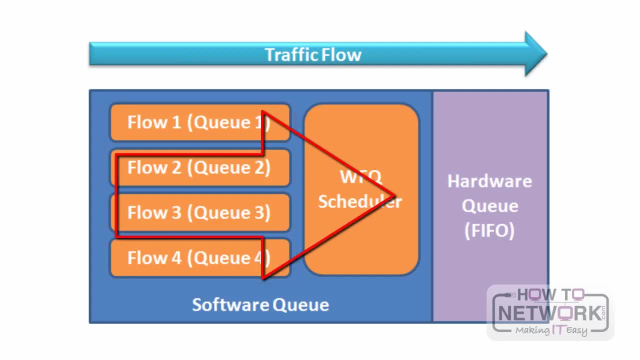 into different queues before entering the weighted fare queue scheduler, which will then allow them to pass to the hardware queue. based upon the defined logic, If one queue fills, the packets will be dropped, but this will also be based on the weighted fare queue approach. 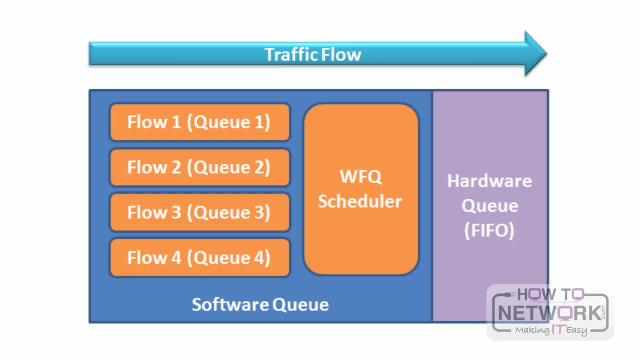 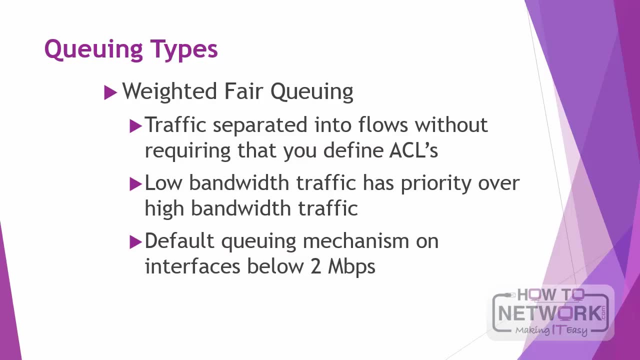 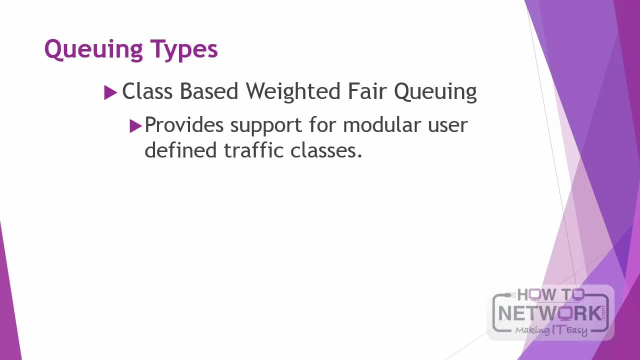 That is, lower priority packets are dropped first, as opposed to the first in, first out approach of tail dropping. Next is class based weighted fare queuing. It extends weighted fare queuing capabilities by providing support for modular, user defined traffic classes. Class based weighted fare queuing lets you define traffic classes that correspond to. 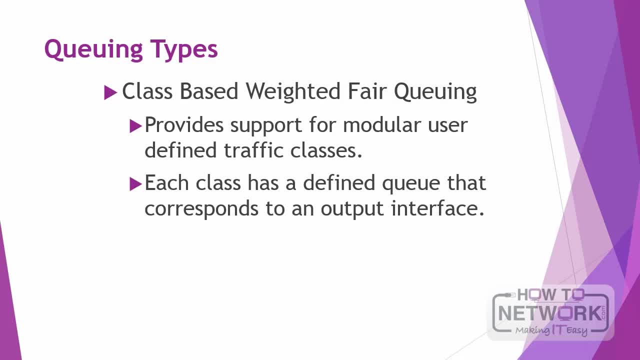 match criteria, including ACLs, protocols and input interfaces. Traffic that matches the class criteria belongs to that specific class, and each class has a defined queue that corresponds to an output interface. So after traffic has been matched and belongs to a specific class, you can modify its characteristics. 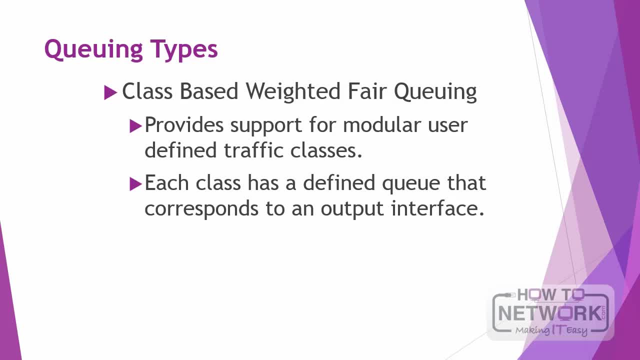 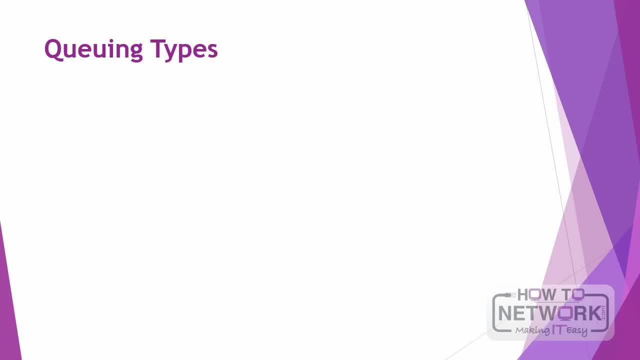 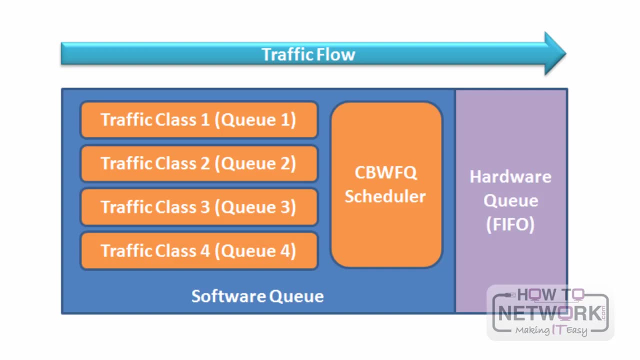 such as assigning bandwidth, maximum queue limit and weight. As you see in the picture here, certain classes- Classes- receive higher priority than other classes. As you can see here. class based weighted fare queuing logic is based on the class based weighted fare queue scheduler that receives information from queues defined for different 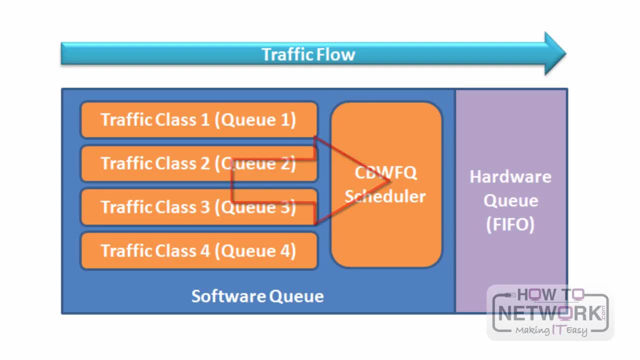 forms of traffic. The traffic that does not fit any manually defined queue automatically falls into the class default queue. These queues can be assigned minimum bandwidth guarantees for all traffic classes. Class based weighted fare queuing offers powerful methodologies for controlling exactly how much bandwidth these various classifications will receive. 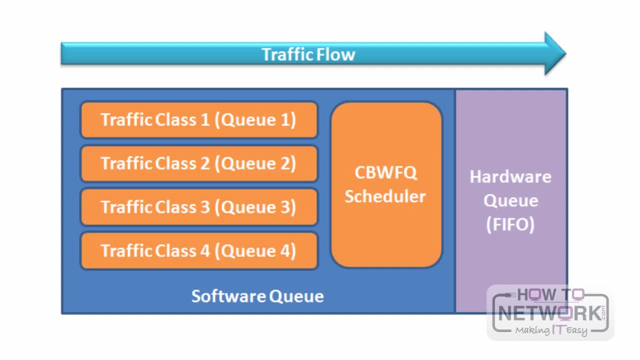 If it contains more than one traffic type, each individual queue will use the first in, first out method inside the hardware queue. So the network designer should not combine too many forms of traffic inside of a single queue, Considering the inefficiency of class based weighted fare queuing. 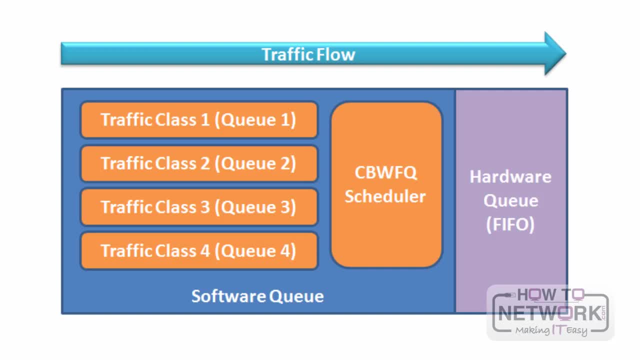 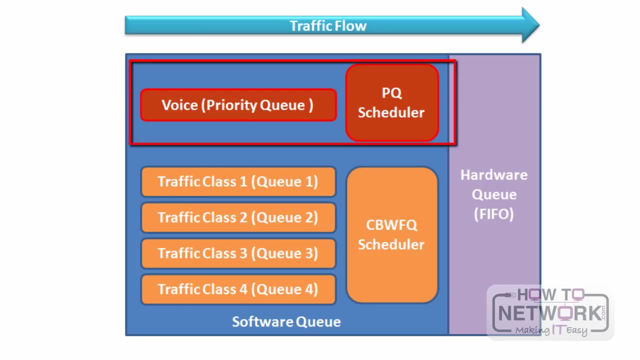 When using VoIP, another quality of service technique was developed, and that is low latency queuing. Adding a priority queue to class based weighted fare queuing will not lead to starvation, because this queue is policed so that the amount of bandwidth guaranteed simply for voice cannot. 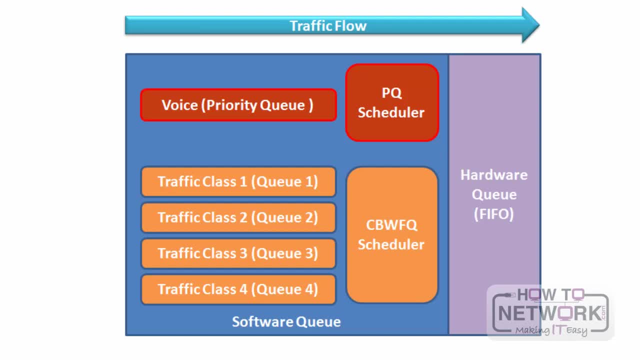 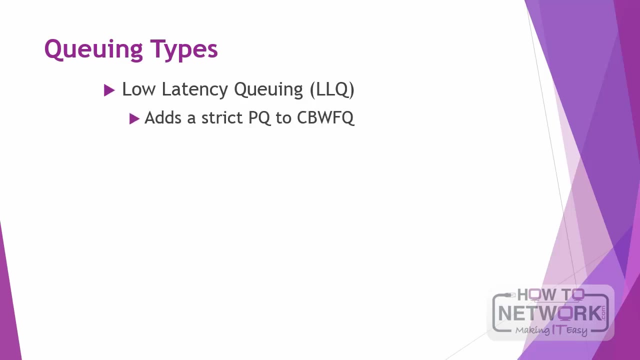 exceed a particular value. Since voice traffic gets its own priority treatment, the remaining traffic forms will use weighted fare queuing based on bandwidth. The priority queue will be set to a maximum threshold on the priority queue and this will prevent lower priority traffic from being starved by the priority queue. 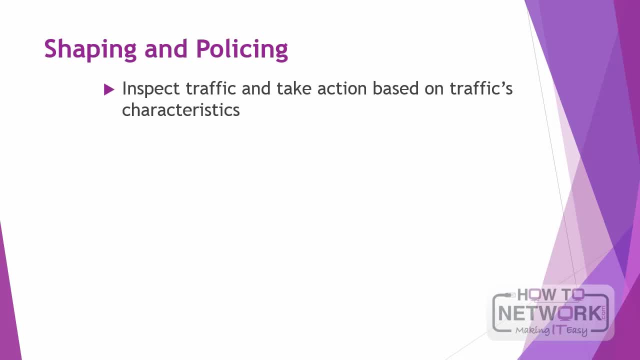 Now that we've talked about queuing, let's talk about traffic shaping and policing. Traffic shaping and policing are mechanisms that inspect traffic and then take action based on the traffic's characteristics. The traffic is shaped based on the traffic's characteristics. It is typically set in the IP header: forests and elements where traffic is sent to a specific 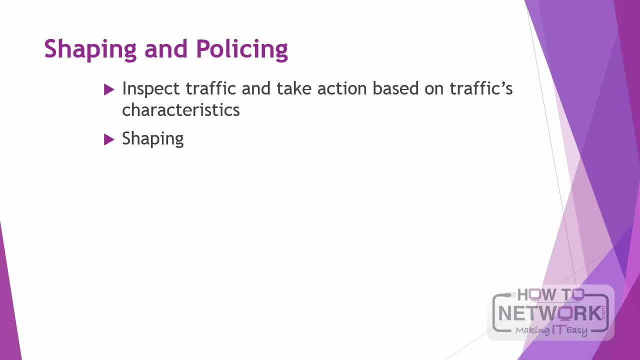 point on the queue. Traffic shaping is a technique in which a pocket is placed to a target point on the queue. Traffic shaping slows down the rate at which packets are sent out at interface by matching certain criteria. Traffic shaping uses a token bucket technique to release the packets into the output queue. 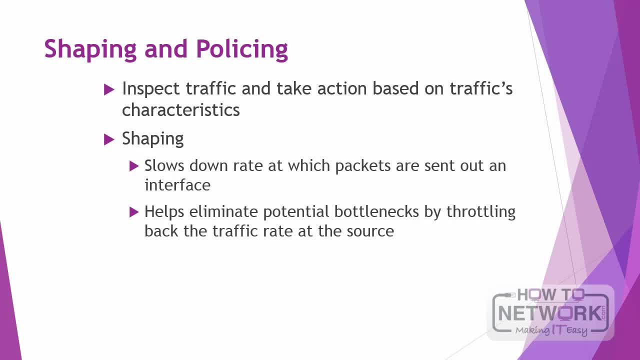 at a pre-configured rate. This helps eliminate potential bottlenecks by throttling back the traffic rate at the source. This method of shaping will be used by a local company. The traffic shaping is used on larger networks, in particular, applications such as DCP IP. 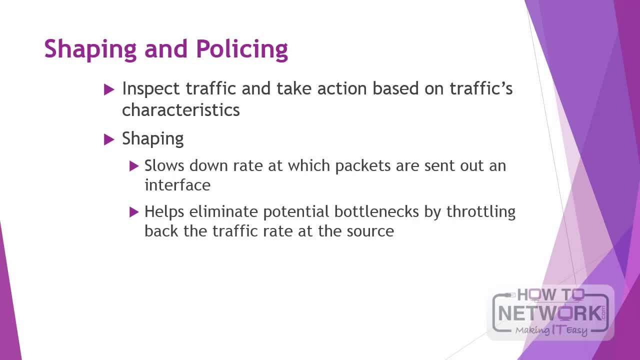 on larger networks to smooth the flow of traffic going out to the provider. This is desirable for a few reasons. In provider networks, it prevents the provider from dropping traffic that exceeds the contracted rate. Now policing is a little bit different, because it tags or drops traffic depending on the